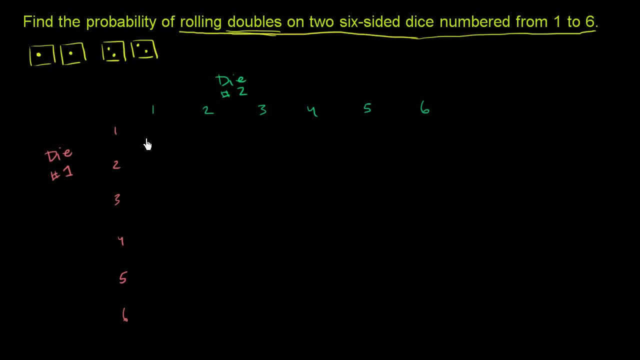 Now, given these possible outcomes for each of the die, we can now think of the outcomes for both die. So for example, in this, let me draw a grid here, just to make it a little bit neater. So let me draw a line there, and then 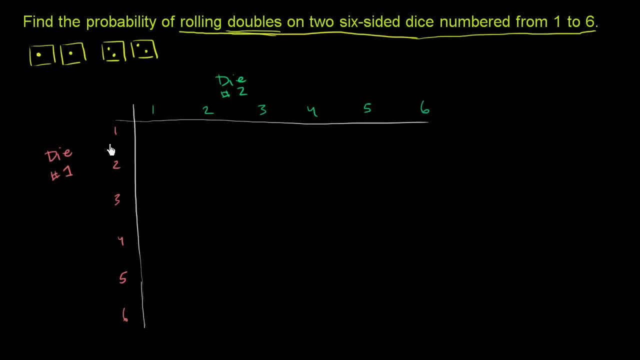 a line right over there. Let me draw actually several of these, just so that we can really do this a little bit clearer. So let me draw a full grid, All right, And then let me draw the vertical lines. Only a few more left. 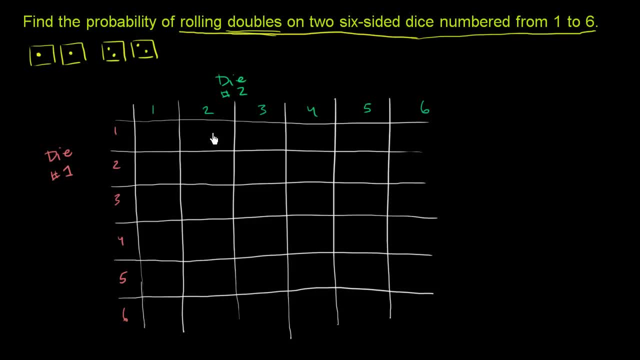 There we go Now, all of this top row. these are the outcomes where I roll a 1 on the first die. So I roll a 1 on the first die. These are all of those outcomes And this would be. I run a 1 on the second die. 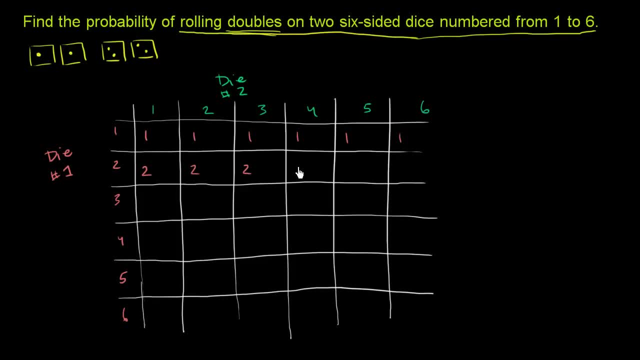 But I'll fill that in later. These are all the outcomes where I roll a 2 on the first die. This is where I roll a 3 on the first die. 4, I think you get the idea- on the first die. 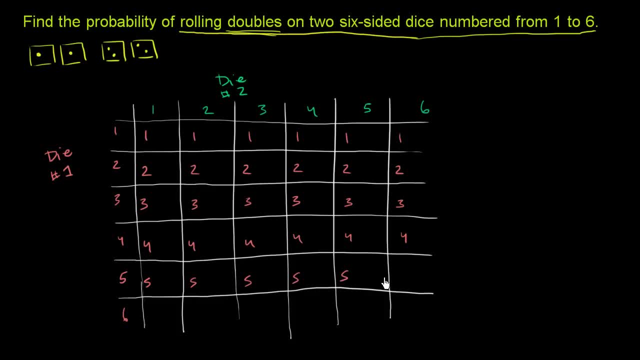 And then a 5 on the first die, 5.. And then, finally, this last row is all the outcomes. These are all the outcomes where I roll a 6 on the first die. Now we can go through the columns, And this first column is where we roll a 1 on the second die. 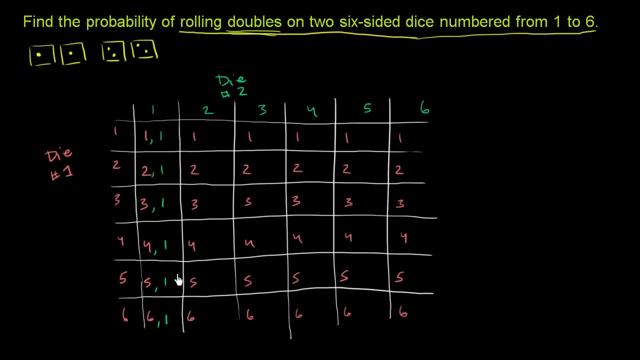 A 1 on the second die. This is where we roll a 2 on the second die. So let's draw that out, write it out, fill in the chart. Here's where we roll a 3 on the second die. This is a comma that I'm doing between the two numbers. 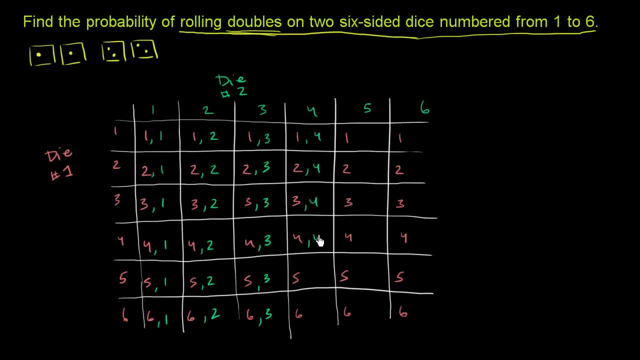 Here's a comma. Here's a comma. Here's where we have a 4.. Here's where we have a 4.. And then here's where we roll a 5 on the second die Just filling this in. Oh, whoops. 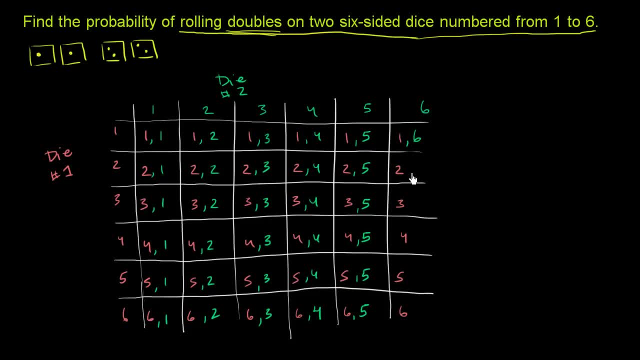 This last column is where we roll a 6 on the second die. Now, every one of these, This last column, represents a possible outcome. This outcome is where we roll a 1 on the first die and a 1 on the second die. 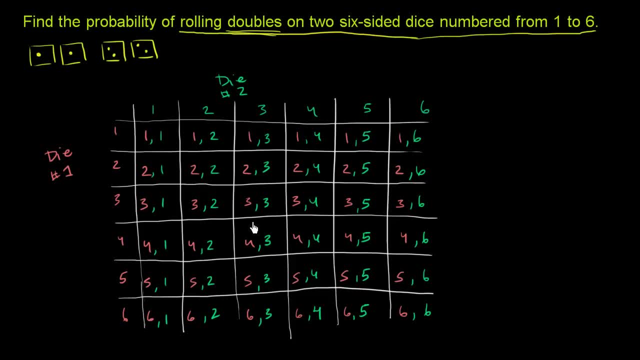 This outcome is where we roll a 3 on the first die, a 2 on the second die. This outcome is where we roll a 4 on the first die and a 5 on the second die, And you can see here there are 36 possible outcomes. 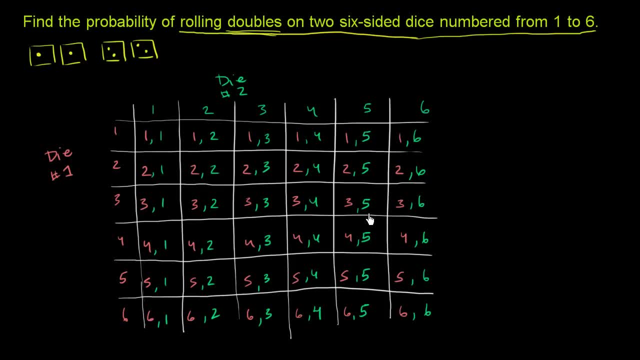 6 times 6 possible outcomes. Now, with this out of the way, how many of these outcomes satisfy our criteria, Satisfy the criteria of rolling doubles on two six-sided dice? How many of these outcomes are essentially described by our event? 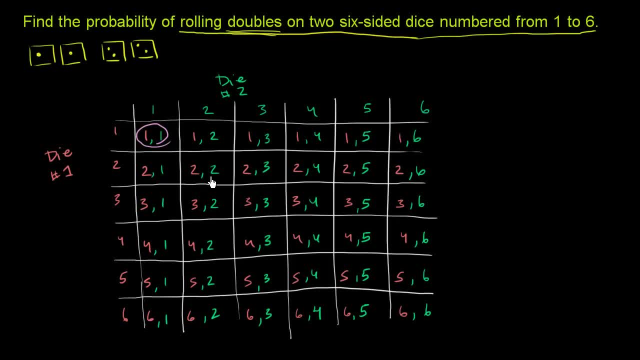 Well, we see them right here Doubles. well, that's rolling: a 1 and a 1.. It's a 2 and a 2, a 3 and a 3, a 4 and a 4, a 5 and a 5,. 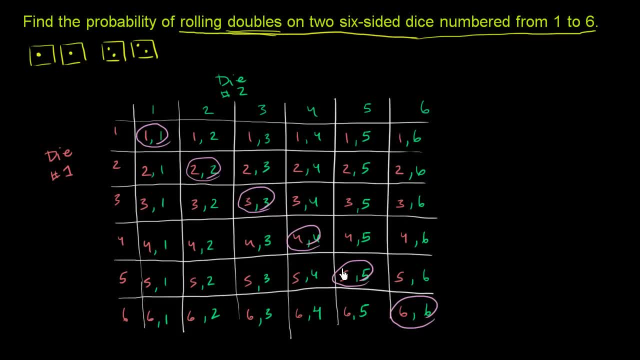 and a 6 and a 6.. So we have 1,, 2,, 3,, 4,, 5, 6 events. satisfy this event or are the outcomes that are consistent with this event? Now, given that, what is the outcome? 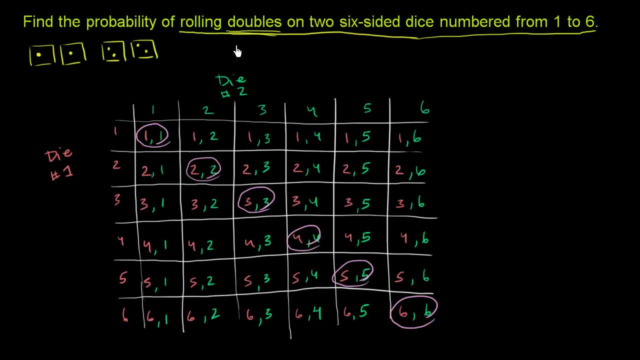 Let's answer our question. What is the probability of rolling doubles on two six-sided die numbered from 1 to 6?? Well, the probability is going to be equal to the number of outcomes that satisfy our criteria, or the number of outcomes for this event, which are 6..